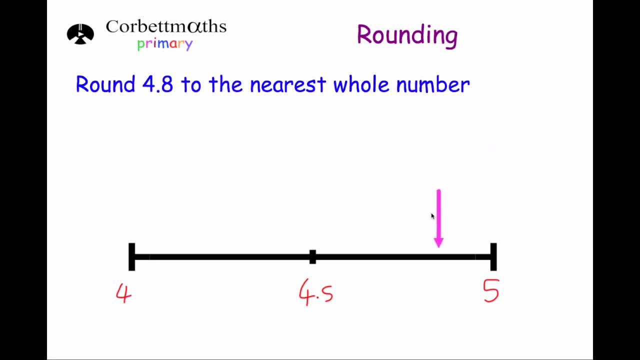 So if we were to place 4.8 on that number line, it would be up here somewhere, because 4.8 is bigger than 4.5. So that means that 4.8 is closer to the number 5 than it is to the number 4.. 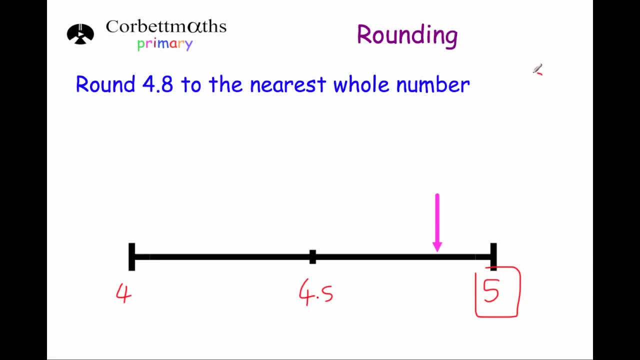 So if we were asked to round 4.8 to the nearest whole number, our answer would be 5.. Right, our next question, Our next question, asks us to round 11.4 to the nearest whole number. So the whole number below 11.4 would be 11 and above 11.4 would be 12.. 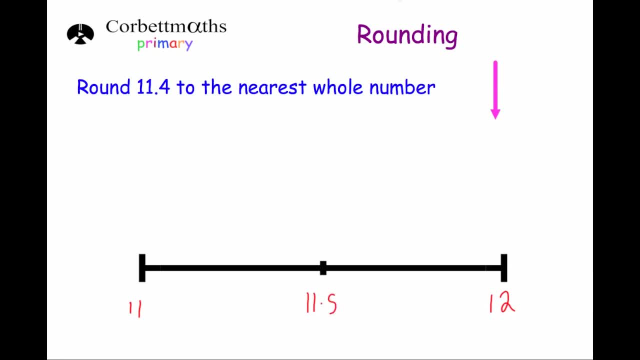 And the midway between those two numbers would be 11.5.. So if we were asked to put 11.4 on the number line, it would be here somewhere It would be below 11.5.. So that means that 11.4 is closer to 11 than it is to 12.. 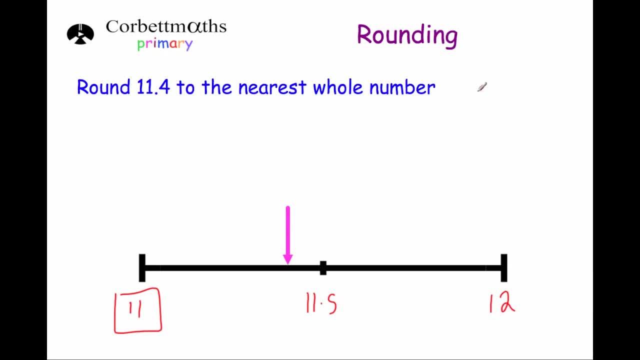 So that means if we were asked to round 11.4 to the nearest whole number, our answer would be 11.. Okay, our next question. Our next question asks us to round 15.6 to the nearest whole number. So the nearest whole number below 15.6 would be 15 and above 15.6 would be 16.. 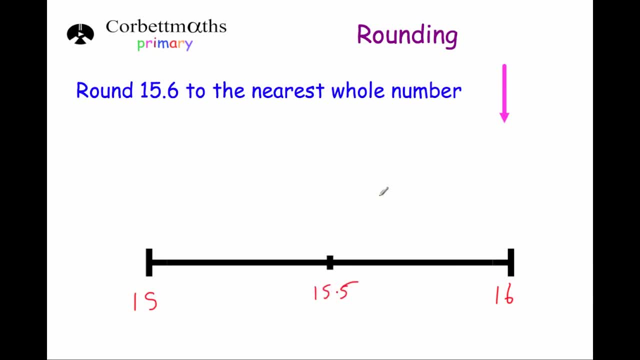 And midway between those two numbers would be 15.5.. So if we were asked to put 15.6 on this number line, it would be around about here somewhere because it's bigger than 15.5.. So that means that 15.6 is closer to 16 than it is to 15.. 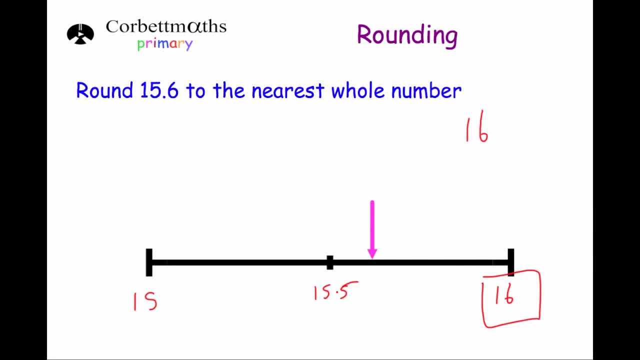 So our answer would be 16.. Okay, our next question. Okay, our next question asks us to round 23.5 to the near sole number. So the near sole number below 23.5 would be 23 and above would be 24, and in the middle is 23.5.. 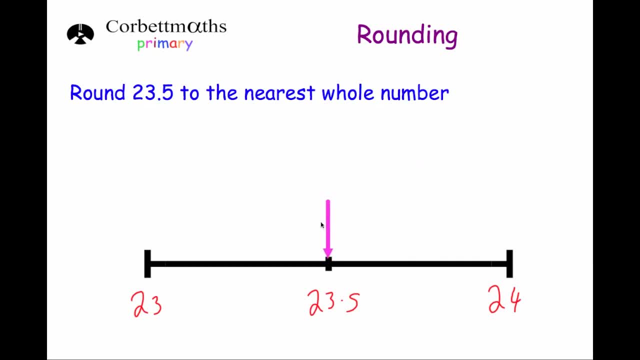 So if we're asked to put it on the number line, we put it here exactly in the middle, because 23.5 is in the middle. Now, if I asked you which number is 23.5 closer to? well, it's not closer. 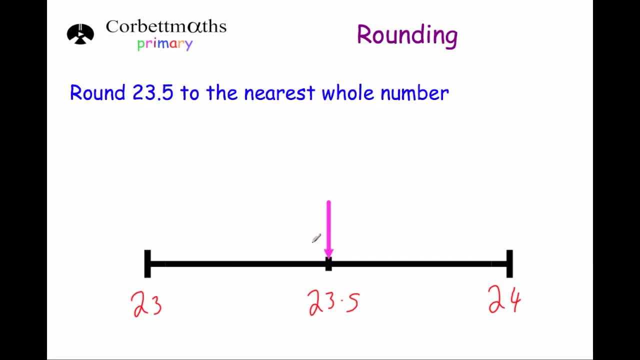 to even number. but the rule is, whenever you're asked to round 23.5 or a number in the middle, whenever you're asked to round that to the near sole number, you round up. Okay so, even though it's not necessarily closer to the 24th and 23,, it's the rule. So if the number is exactly in the